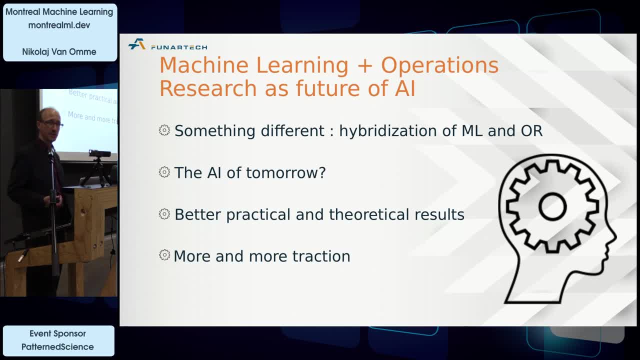 OR is operations research or operational research. By the way, who knows a little bit or knows about OR? Wow, A lot of people. Great. So what we are doing is combining ML, machine learning and OR. From now on We say ML, it's machine learning OR operations research. 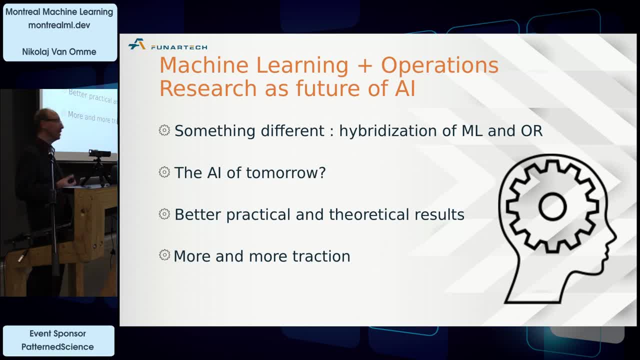 So why do we think it's the AI of tomorrow? Well, the thing is, we have better practical and theoretical results, So that's a good hint that it might be something useful. Also, we get more and more traction, or that idea get more and more traction. 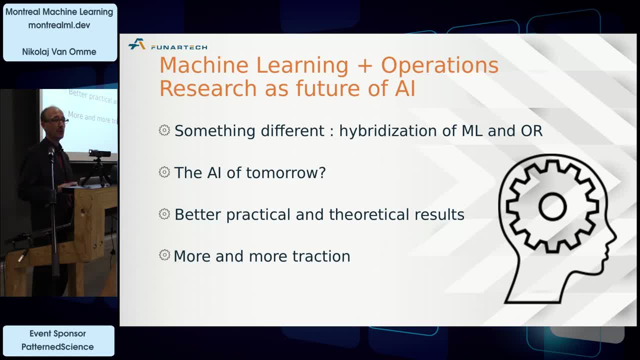 And, as I said, one of the way to combine ML and OR- sorry- became mainstream this year. So when I'm talking about ML, I'm talking about AI, I'm talking about AI, I'm talking about AI, I'm talking about automation. 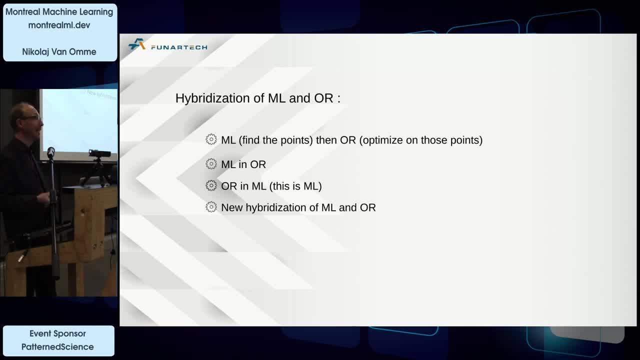 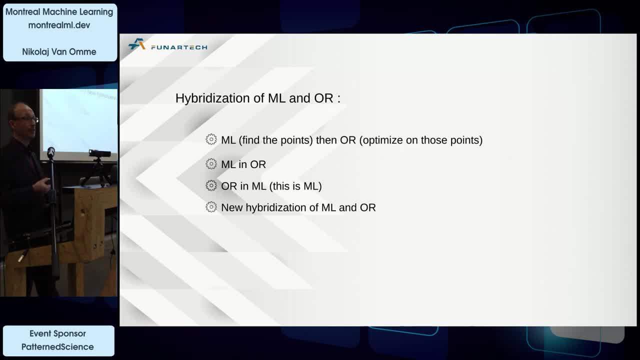 Basically, you can combine ML and OR in four ways. The first one, which is becoming mainstream this year, is to combine ML and OR as black boxes. So you use one and you use the other, but separately, And most of the time you use first ML to predict and then you use OR on those predictions. 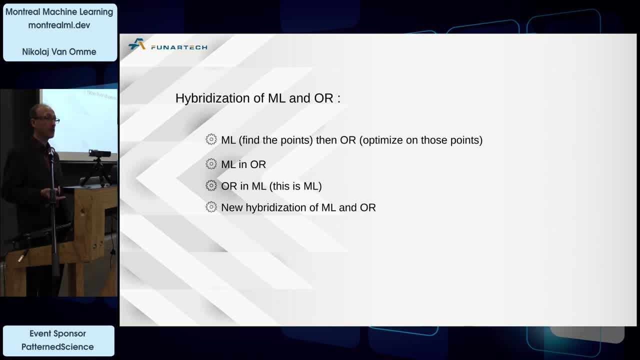 to optimize. So what we're going to do is we're going to combine ML and OR in four ways. Okay, you can also use one to improve the other. so you can use ML to improve OR works very well. you can also use OR to improve ML. actually, this is what ML is. 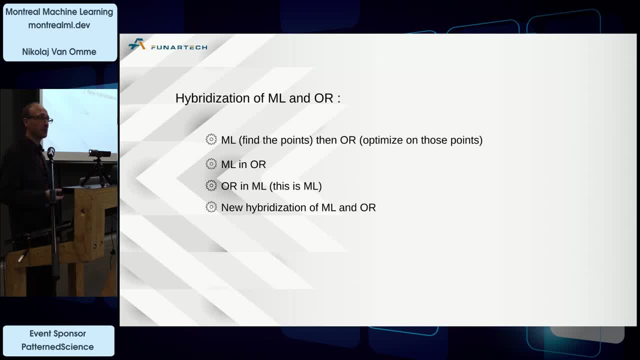 because OR- I'm gonna talk a little bit more about OR in a few seconds- but OR is basically the science of optimization. whenever you talk about optimizing something, I want to minimize, I want to maximize something. actually, there is a science behind this and it's OR operation research. so ML is basically. 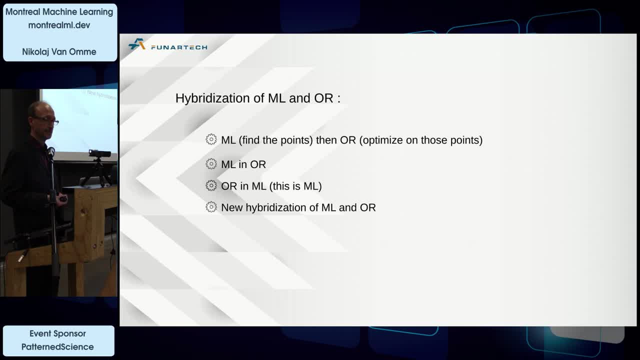 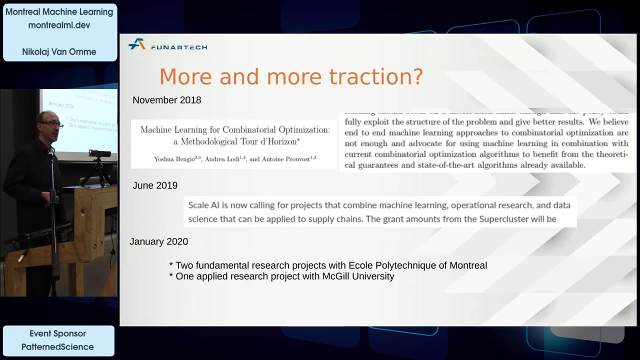 using operation research to optimize its prediction. and then there is this new way of doing things, a total, complete hybridization of both, where we have new algorithms, and I'm going to show you two examples of things you can do with that hybridization. so more and more traction. yes, well, I'm gonna use the mouse. so in 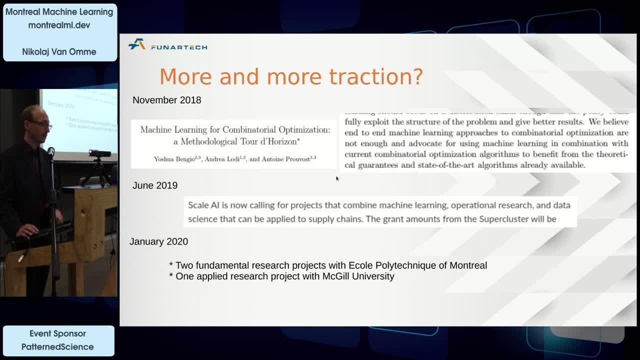 November 2018. so I have three examples here. you can see that I have two algorithms here and I have three algorithms here, but there are lots more machine learning for combinatorial optimization and methodological methodological tour d'horizon from Joshua Bengio. 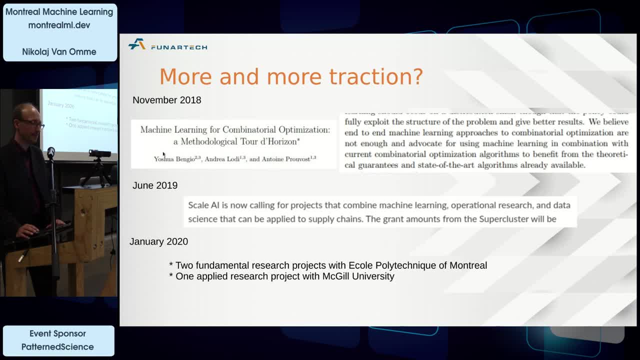 Andrea Lodi and Antoine Prouveau- I guess you know at least the first one. so this is a review and this is the conclusion. and in the conclusion I'm gonna read: we believe end-to-end machine learning approaches to combinatorial optimization are not enough and advocate for using machine learning in 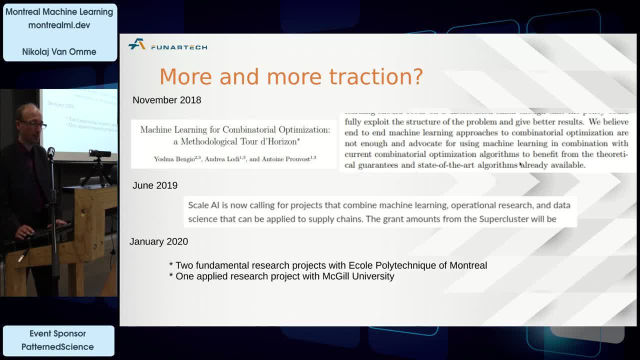 combination with current combinatorial optimization algorithms. to blah blah blah. combinatorial optimization is OR, so in that article they say literally: use ML and OR for combinatorial problems. June 2019, scale AI, one of the five big clusters in Canada, scale AI is now. 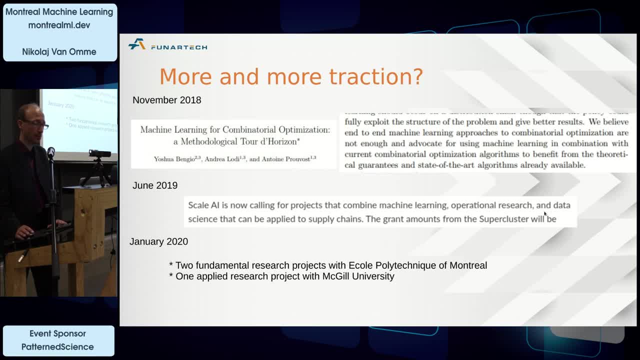 calling for projects that combine machine learning, operational research- again OR- and data science that can be applied to supply chain ourselves- Fanartech in January 2020. in 2020, we're going to start two fundamental research projects at Ecole Polytechnique and we're going to start an applied project at McGill. there are 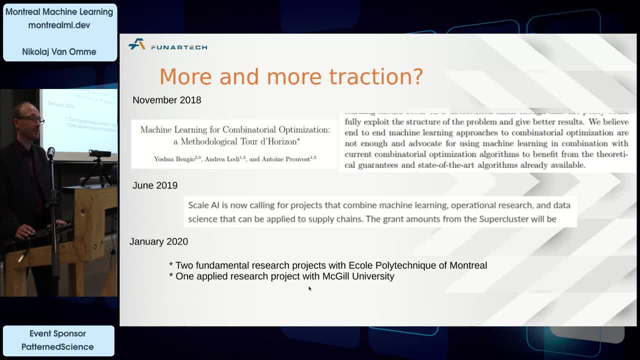 lots of other examples of that. the combination of ML and OR is really becoming mainstream. by the way, I don't know if you noticed- on the sixth presentation today, there are three proposing to combine ML with something else, and actually that's the future, because ML is great but it's also not. 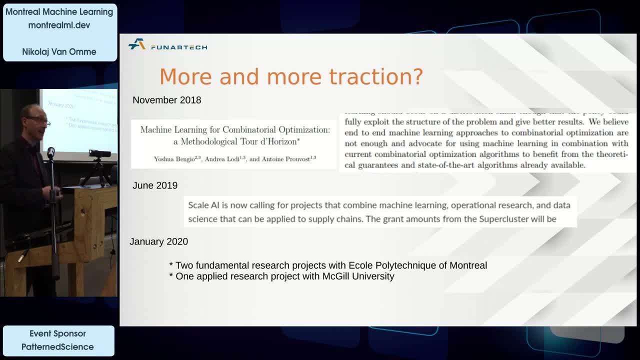 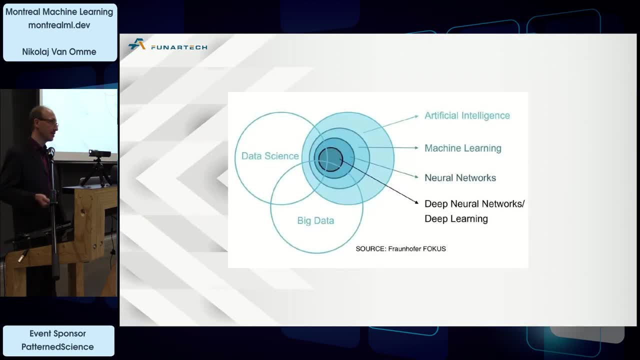 Hb2, it's great, but if you, if you combine it with something else, you have even better results. so that's the big picture in general when you talk about artificial artificial intelligence. so you have artificial intelligence and inside artificial intelligence you have machine learning and we need machine. 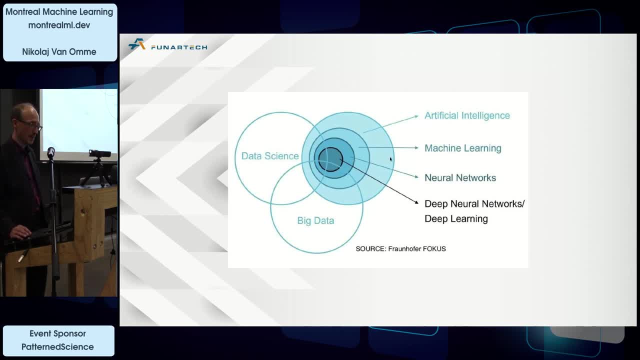 learning, you have deep learning. that's the picture we usually see. in fact, there are some candidates missing, and in particularly, there's this one missing. it's- OR actually all those fields- are based also on data science. the data learning project is different, because data science is not a problem when it's. 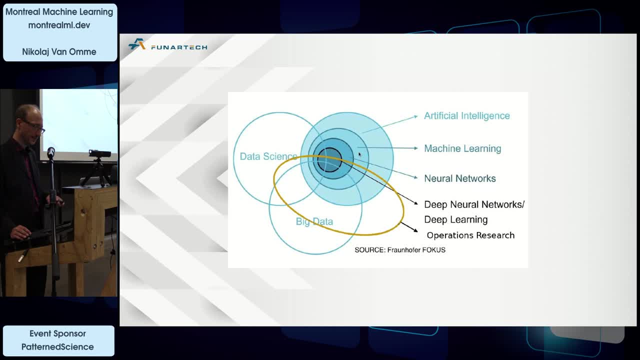 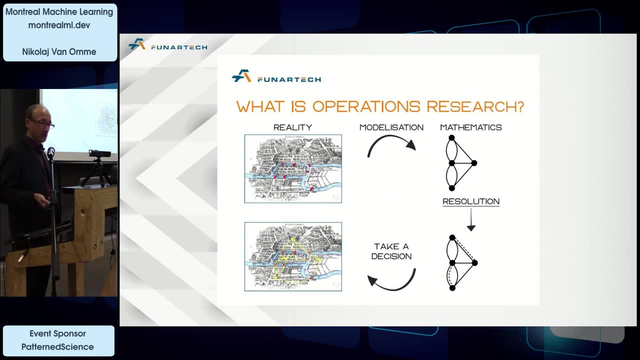 possible to do so in the future. in the future, it will be a problem, no matter how, on or up to a point. so what is? or? so, as i said, it's the science of optimization, how do we use? or well, basically, it's always the same way to do things. we have a real problem like 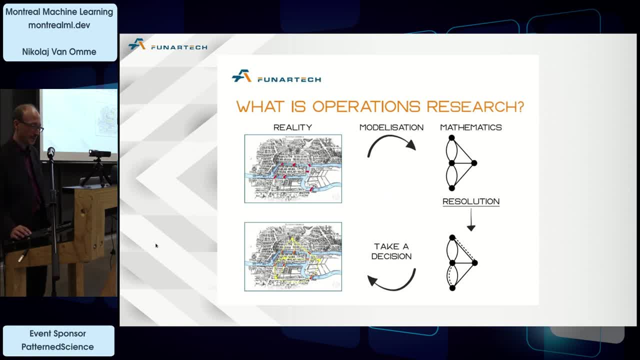 here we have the problem of crossing bridges in a city, so we have seven bridges, so it's a real problem. i'm gonna talk about it a little bit later. and then we modelize that problem into a mathematical model. we solve that mathematical model mathematically. we find mathematical. 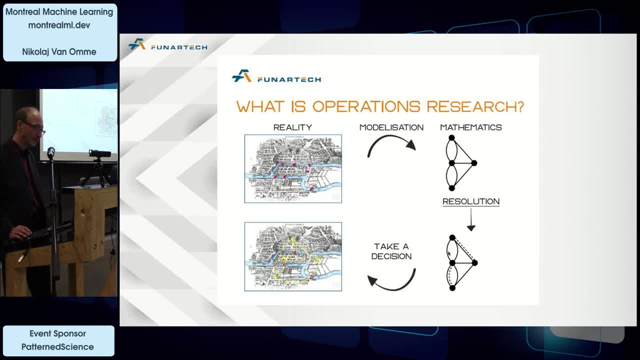 solutions and then you try to translate those solutions back into reality to be able to take a decision. by the way, if you know prescriptive analysis, this is done mostly by or while ml is doing predictive analysis. so here, for instance, you have seven bridge in a city called kaliningrad. now, 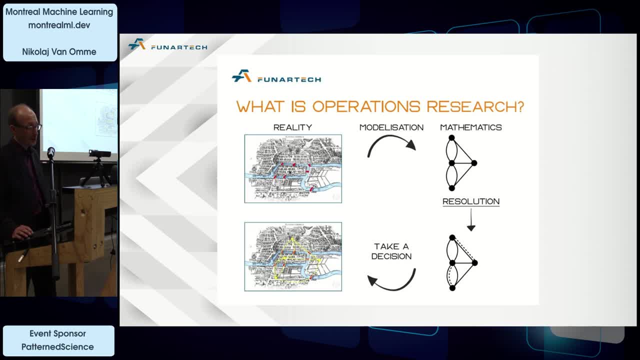 it's um, i mean it's now kaliningrad. it was going to born Carolina where there was banner of maldon ladies, not mald, hosting their good luck, nice. one way to solve that problem is to modulize this into a graph where actually a bridge is replaced by an edge. so the question now becomes: can i do a tour in this? graph by crossing each edge only once. by the way, this is a graph. graph theory is part of, or. the solution is no, it's not possible. so there is another question. okay, i need to find something. answer to this quick problem. you don't really know this. that is a very choppy翻. Swine 1000. 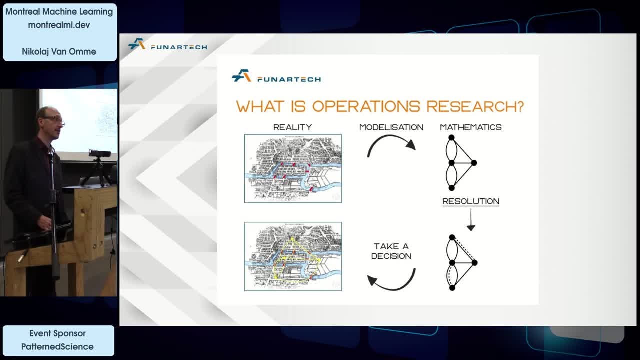 question, which is exactly why we have a lot of unemployment. you didn't find anywhere in the midwest where the interactions that are not currently considering, for studying, for example, need absolutely to cross a bridge, at least twice. how many bridges do I need to cross minimally? 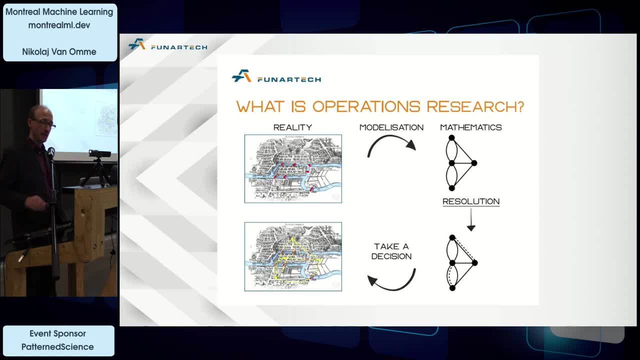 to be able to do the tour? The answer is two. We can prove this mathematically. Here you have a solution And then, in this case, it's quite easy to translate that solution back into reality. But most of the time, doing that translation back. 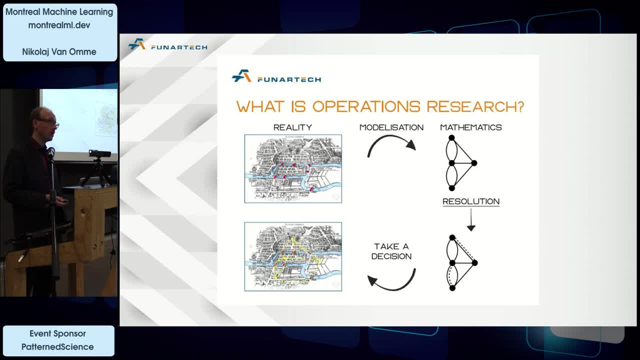 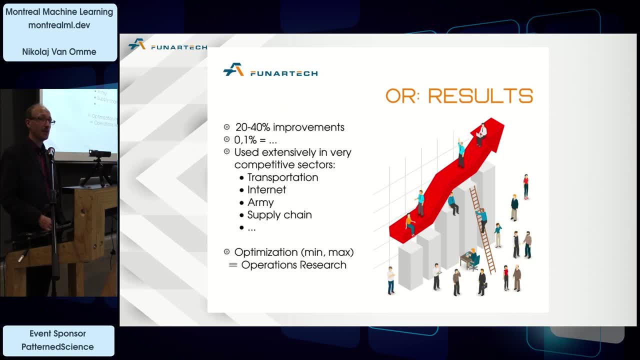 is not that easy. So that's basically what we do in, OR Some results We get often, not all the time, but we get often 20%, 40% of improvement. This is huge. In the case we don't and we only get- I don't know. 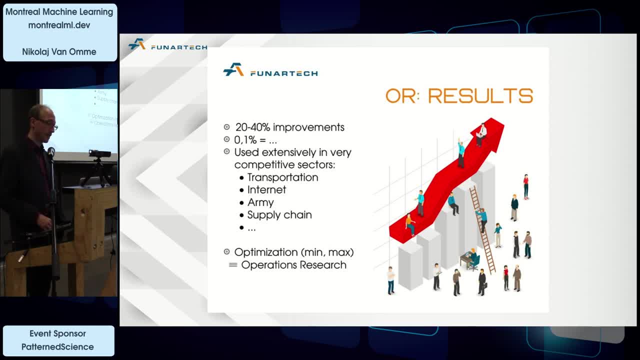 0.1% of improvement, it can still be worth it. For instance, if you can minimize the pollution on Earth by 0.1%, it might be worth. It's already used extensively in a lot of sectors: transportation, internet, RME, supply chain and others. 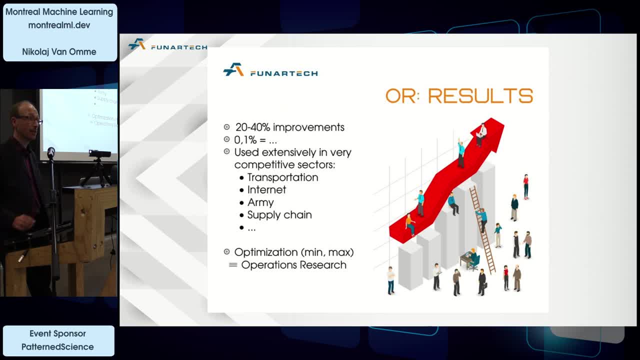 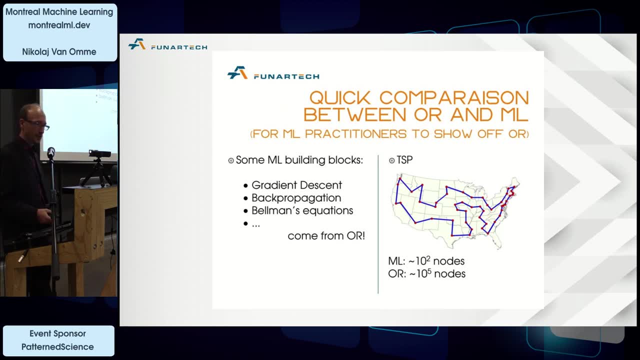 And, as I said, optimization, OR is the science of optimization, Quick comparison between OR and ML just to show off OR. So on the right, you have the TSP. TSP is the Traveling Citizen Problem. That's a problem where you have cities. 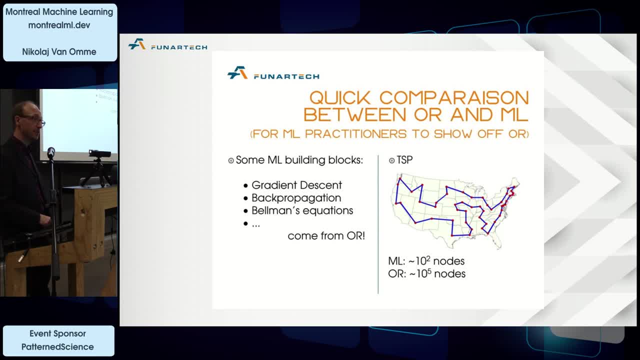 and you want to do a tour, visiting each city only once, And you want to come back and you want to do this for a minimal amount of effort, like, for instance, a minimal distance, minimal time, something like that. It's an NP-hard problem. 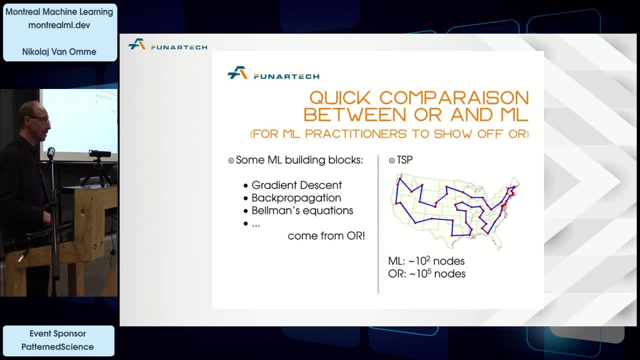 People in ML try to solve that problem and they can solve it today up to 100 nodes, which is great. But look at what OR is able to do. OR is able to solve this with 100,000 nodes. Again, this is an NP-hard problem. 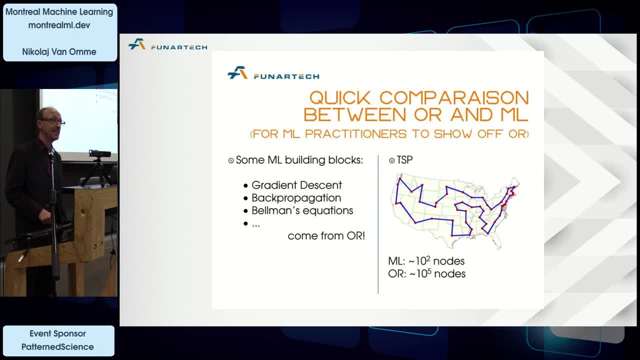 So going from 100 nodes to 200 nodes is already very difficult. Imagine the gap between the two. On the left you see a column where I'm writing that and you see that most building blocks of ML are coming from OR like gradient descent. 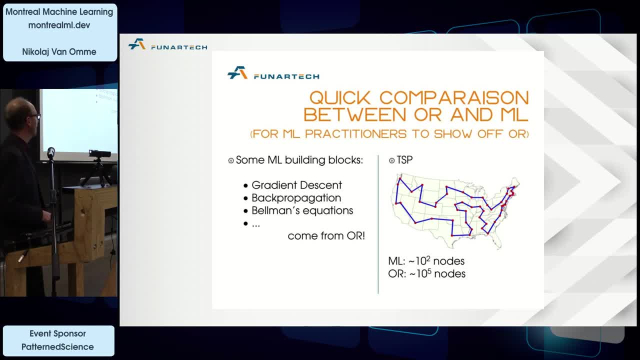 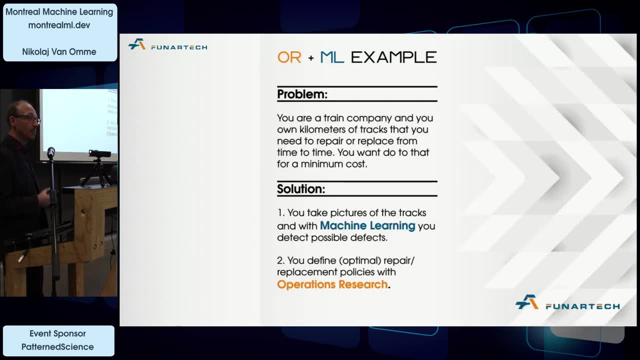 Gradient descent is coming from, OR Even back propagation is coming from, OR Bell-Sman equations, OR, et cetera. Now an example on how to combine them both. This is becoming mainstream this year, So you use them both separately. 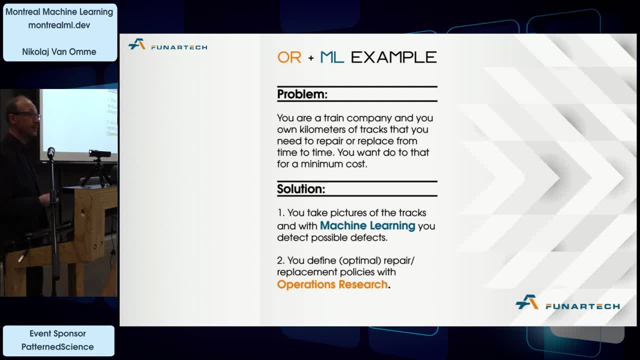 So let's say you're a train company and you want to repair, replace your tracks. How can you do this for a minimal cost? One way to do this is to use the TSP. One way to do this is in two steps. 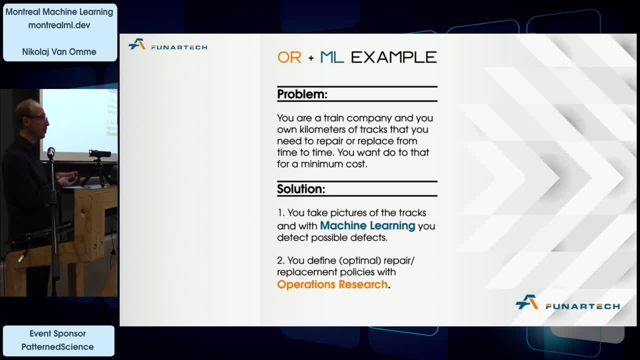 First step: you use deep learning. So you put cameras under your wagons, You let your train go, You take pictures in quick succession. With deep learning, you're going to stitch those pictures And with deep learning, you're going to be able to say: oh, I need to replace that track in three. 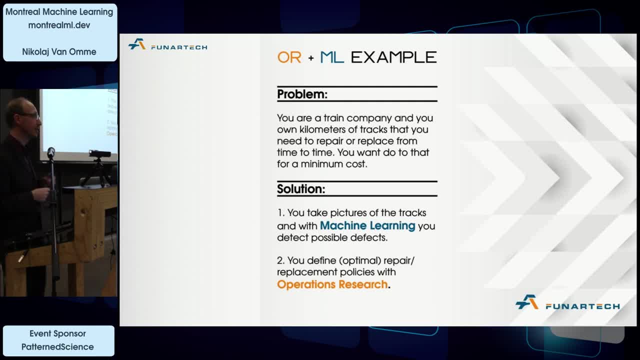 months, this one in six months, this one in two years, These ones need to be repaired, and things like that. You have a mapping of what you need to do, But you don't know how to do it, Because you can send a team to replace. 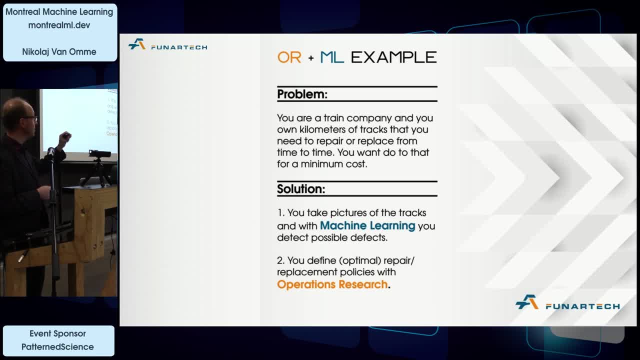 a track, But maybe that same team should also replace or repair another track next to it, even though it shouldn't be repaired right now, maybe in six months or two years. But it would cost less to do it right away than to send again another team later on. 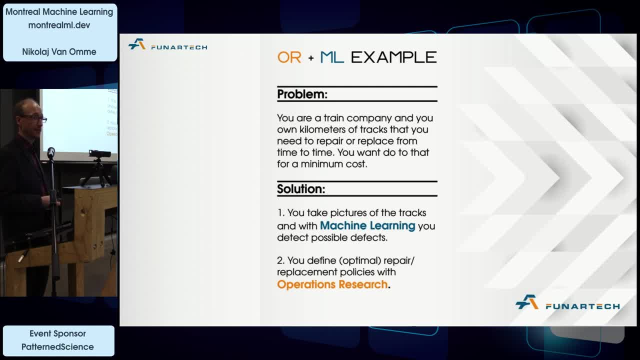 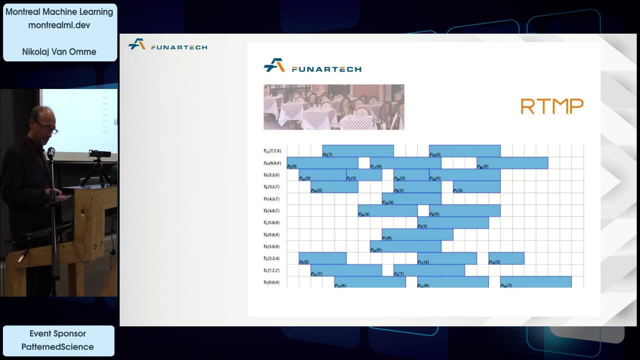 This is what OR can do. It can optimize that. So that's the perfect combination of OR and ML. So with ML you have predictions, With OR you can optimize on those predictions, And time is flying by, And that's an example we did at Funartech. 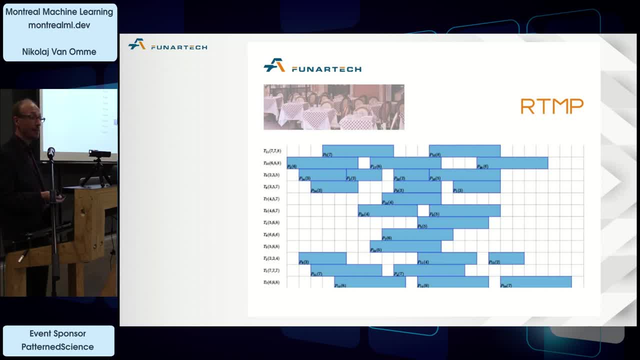 So we had a restaurant chain that asked us to optimize their booking system. So before we came, the way they did it was to have someone calling them, And then they said: OK, what do you need? Well, I'm coming at 6.. 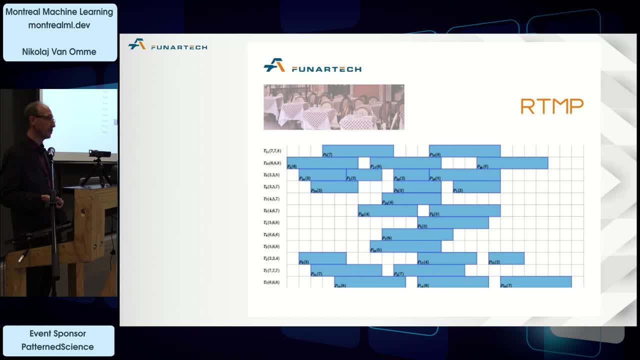 I need a table for 4.. And then you guess it, Because there are four, they're going to stay for two hours. It's a very stochastic problem, because actually they came only three. I mean only three of them. 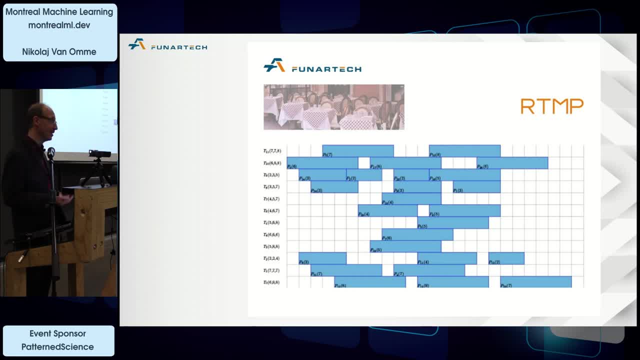 And instead of coming at 6,, they came at 6.20,, for instance, And they didn't stay for two hours, but for four hours. So basically, before we did anything, what happened was the assignment was done and fixed once. 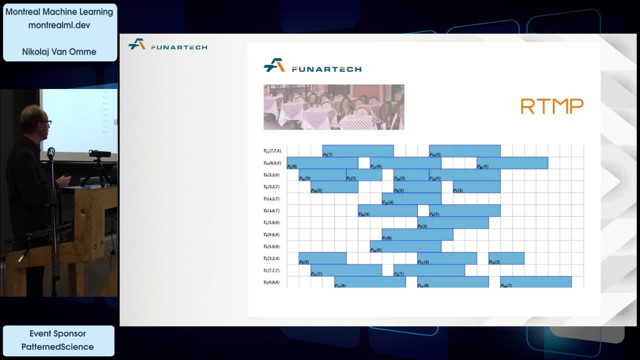 and for all. That's suboptimal, Because it can happen that you are assigning a table of eight to a group of five And if you don't change that, maybe later on this is going to be a group of six And they will not be able to come because that table is. 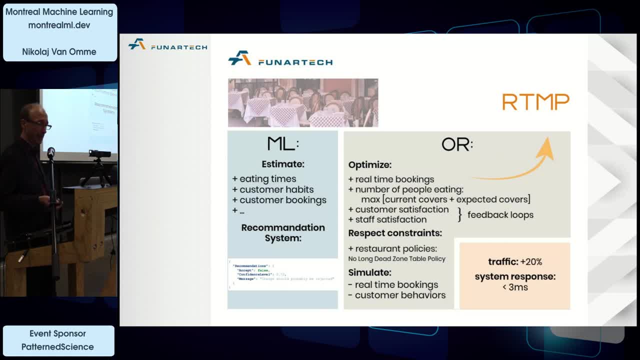 in fact already occupied. So just to tell you that we combined ML and OR, So ML you can optimize, I mean estimate eating times, when they are eating, when they are booking and things like that. We also build a recommendation system telling them OK. 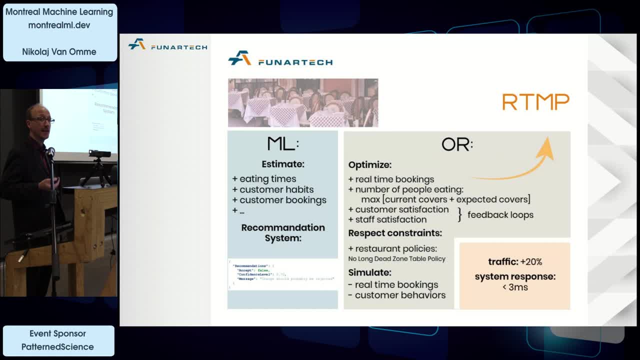 maybe you shouldn't accept a booking, even if that booking is possible, Because there is another one coming after. Or maybe there was someone coming at the door without reservation And you would not be able to accept that group if you accept that booking. 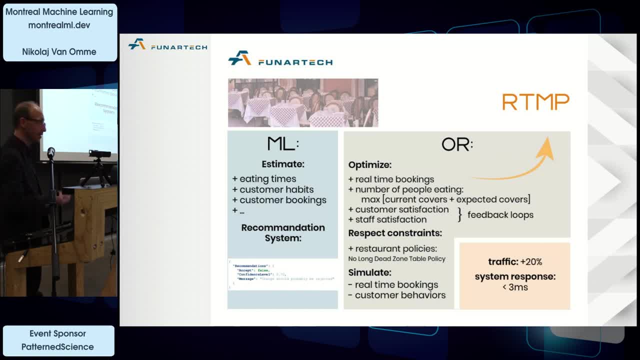 And then we used OR to optimize the overall assignment of tables. We got 20% of improvement. That's huge And, by the way, I'm also very proud that we could do this system under three milliseconds. I mean, the system was reacting under three milliseconds. 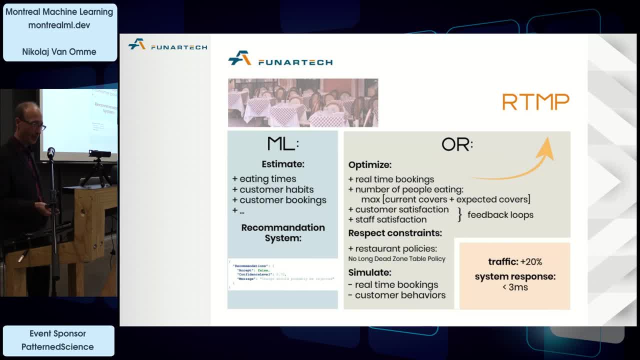 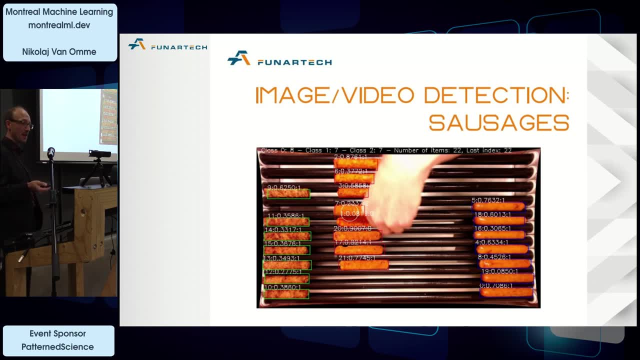 I had something very interesting about the constraints, But the thing is I only have a few minutes left And I would like to talk about the total hybridization First of all. This is another problem where we use ML and OR like two black boxes. 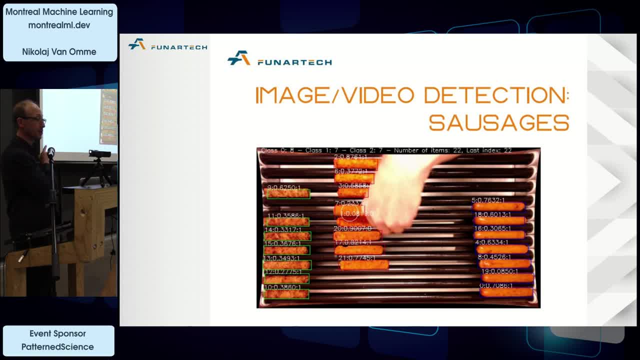 So this is typically a computer vision project where we want to recognize sausages. Just to say that if you use deep learning, it works not that very well Because we had a 2D camera, not a 3D, And people were manipulating the sausages. 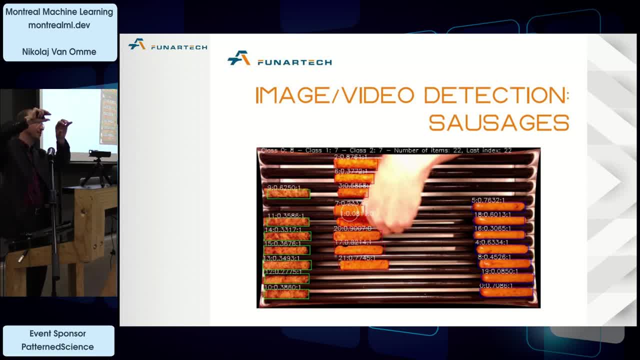 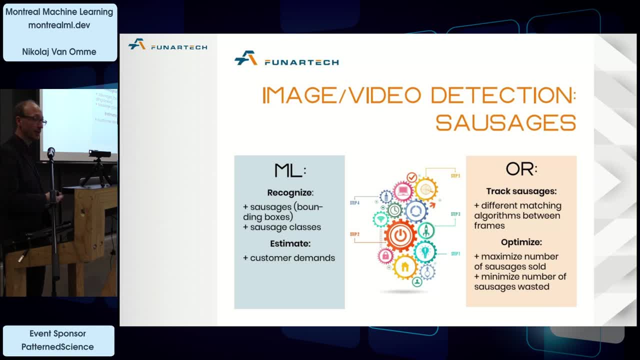 So when you had a sausage and you put a smaller sausage in front of it, the system is totally lost. So deep learning is not working very well. So what we did was to use ML- yes, deep learning, and also OR, And actually we had much better results. 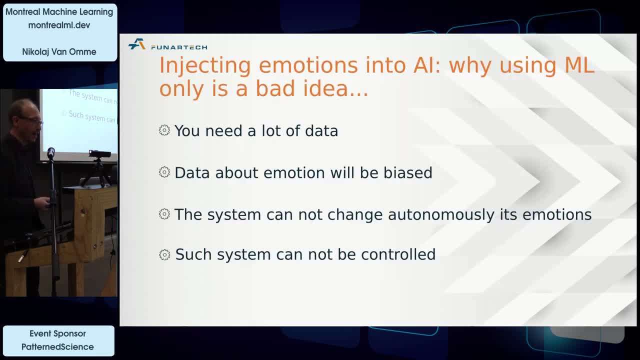 But I don't have time to go over that one Here. I want to take some time about those two projects. So I'm talking about a total hybridization of both, So we have new algorithms. One first project is about injecting emotions into AI. 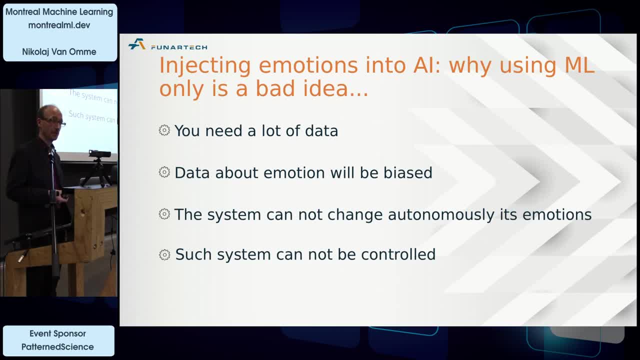 So we are not doing sentiment analysis. We are making the bots emotive, making them angry, happy, empathic, whatever. If you are trying to do this only with ML, there are lots of problems that are popping up. Here I listed four. 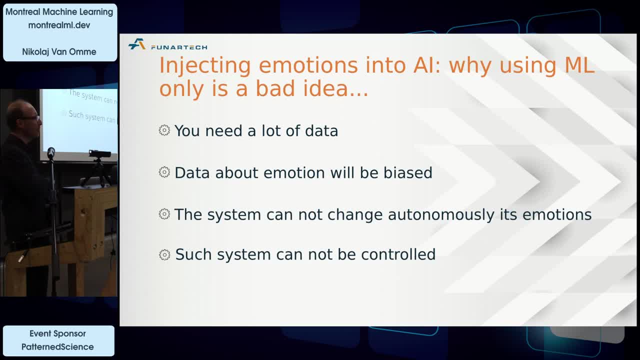 There are many. maybe not many more, but there are some other problems. So, first of all, you need a lot of data. I mean, emotions are really contextual. You need a lot of data. You also have data that will be biased. 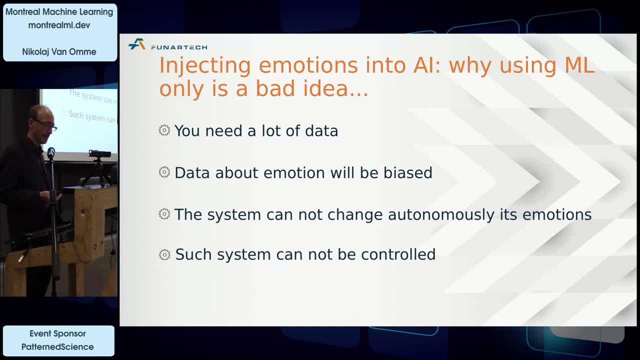 Because emotion. it's really hard to get data. Then the system cannot change automatically its emotion. It's really hard. You need data about it Right, Changing emotion Already. having data about emotion is hard, but about changing emotion is even harder. 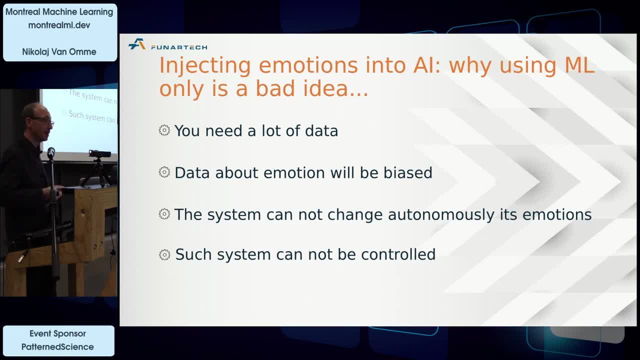 Also. another problem is that such system cannot be controlled. Your system can be totally going berserk. Why am I listing this? It's because we have a solution for that with OR, by combining OR and ML. So if we have data, we use it. 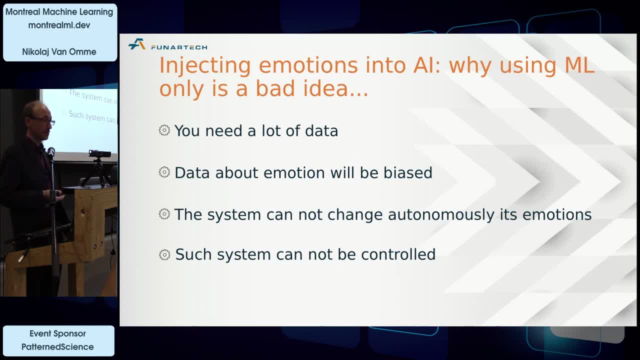 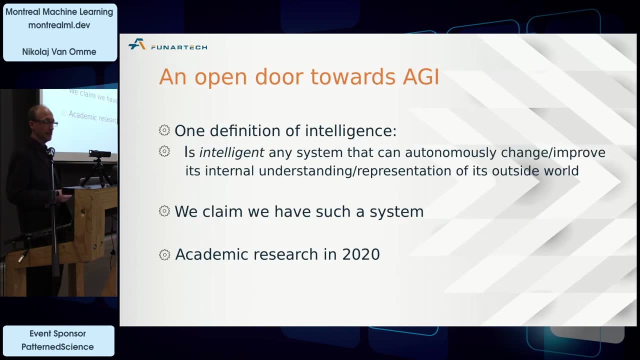 We don't need a lot of data About biases. we have solutions. Our system can change its emotion autonomously And it's totally controlled in the sense that it cannot go berserk. Another project that is even crazier: it's what we call an open door towards AGI. 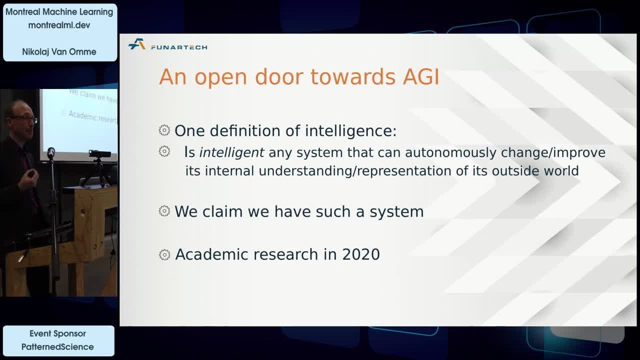 So we don't have AGI, but we have something that maybe might lead to AGI. What we have is the first really truly intelligent algorithm. So when I'm saying this, it's because we're not really mimicking the brain. 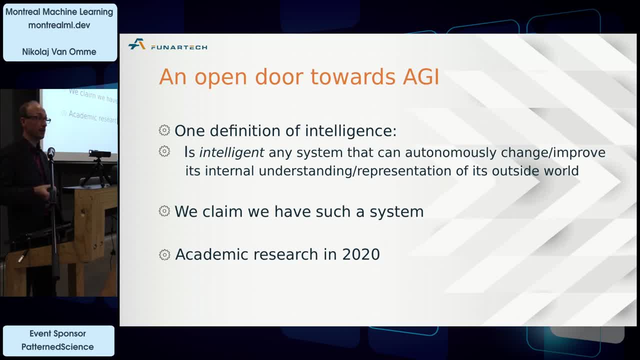 This is way too difficult. We don't believe that we know enough about the brain, on how it's working, So what we do is trying to have a system that you would like to call intelligent, So we have a system that is able to autonomously change. 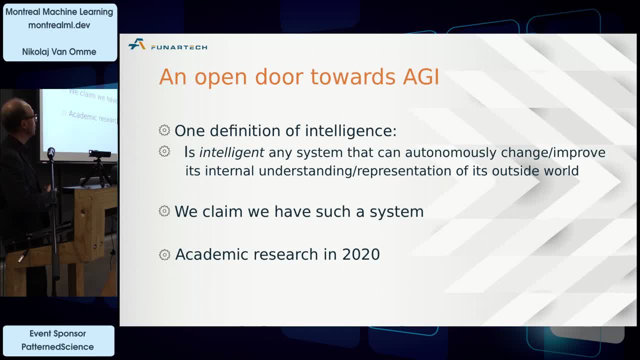 its perception, its learning, its vision of its surrounding in a way that it can improve it, and also that it can totally get rid of what you are giving it at the beginning, So it can erase completely what you're giving the system. We would like to call this intelligence. 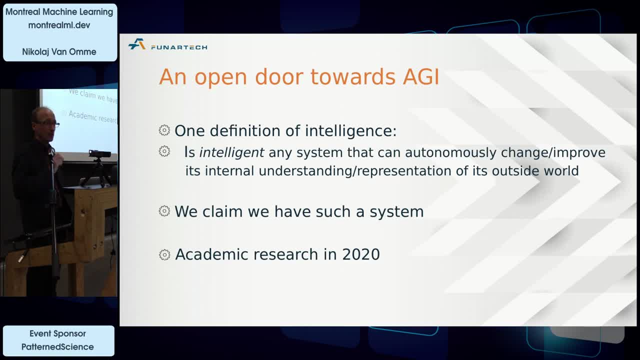 We claim that we have this, Not that we think we know how to get there. No, We claim that we have this. The other problem: we already have code This one. we don't This one. we're going to start January 2020 at Polytechnique. 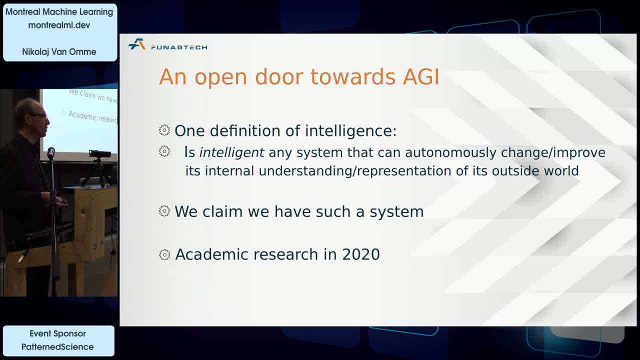 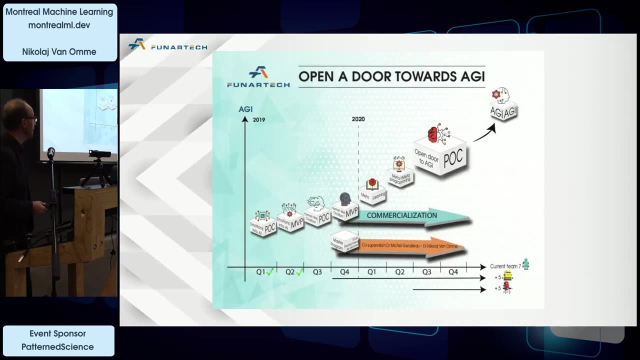 But the thing is we believe that we can make this work, Not tomorrow, but maybe after tomorrow. So that's something you can do with the combination, the hybridization of ML and OR, And this is our roadmap. No idea if we get to AGI, but at least we might get to this. 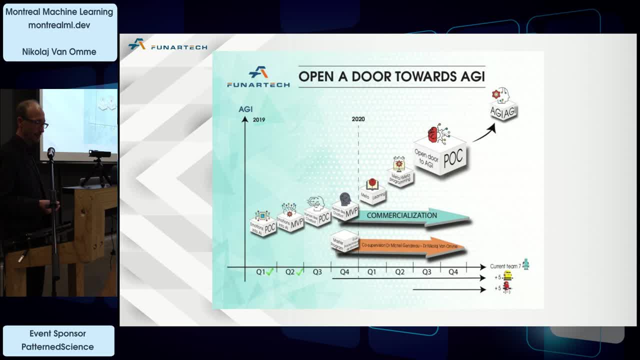 intelligent system. So for the moment we are a little bit late If you look at Q1, Q2, so we did a POC for the emotions into AI, We did an MVP and we showed it, But we are late on the POC. I mean the third step. 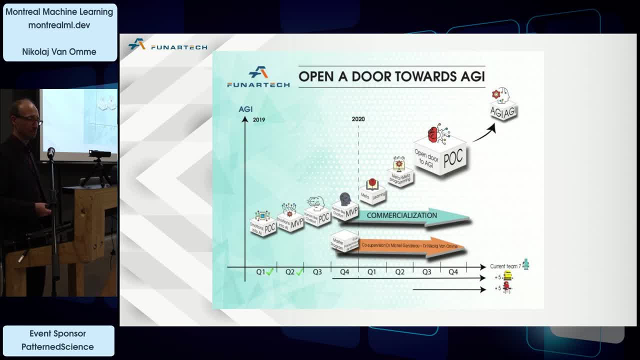 But anyway, we hopefully will get there somehow, And that's it. Thank you very much, Questions. Thank you for your talk. Let's take a break. We want to take a look at the technology behind the OTO system. You call it OTO optimization. 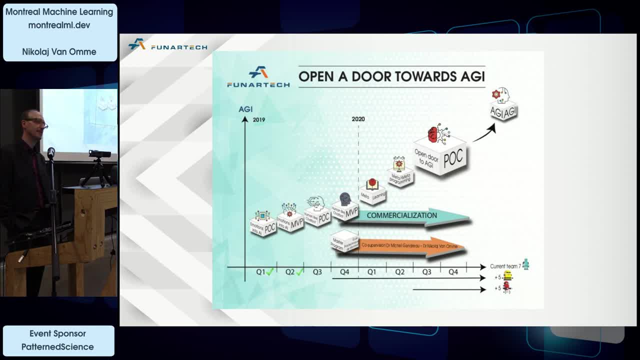 Did you use Cplex OPL? We could have used Cplex, but we don't because it's too costly for us. But yes, we use such tools. if that's the question, Yes, we do. I love this. 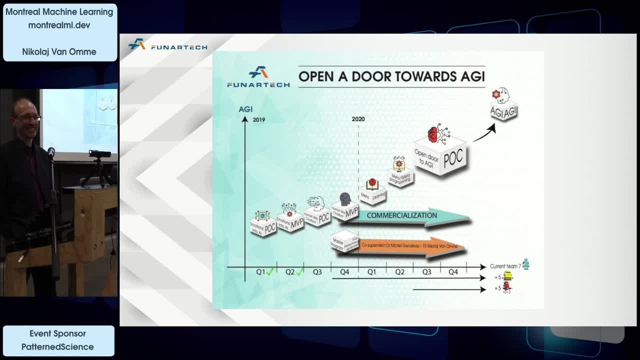 It's such an example. It's perfect, Yes, So how flexible is what you need for changing to another task? that is like vision and you have to keep track of this. What is the degree of freedom you have for it? It's extremely flexible. 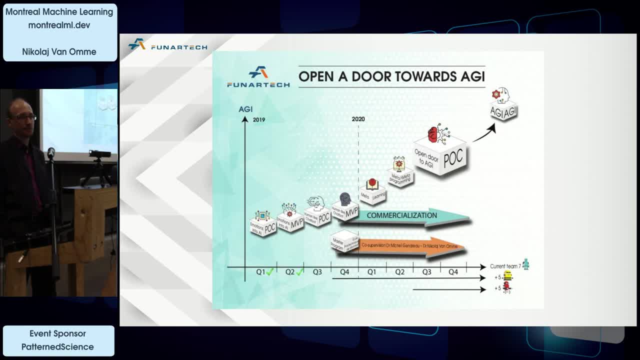 Actually, I truly believe that you can apply this to anything, Anything, Anything. I'm doing this since 25 years. I didn't see a single example where it didn't apply. Okay, So what you're doing is you're doing a very, very robust optimization. 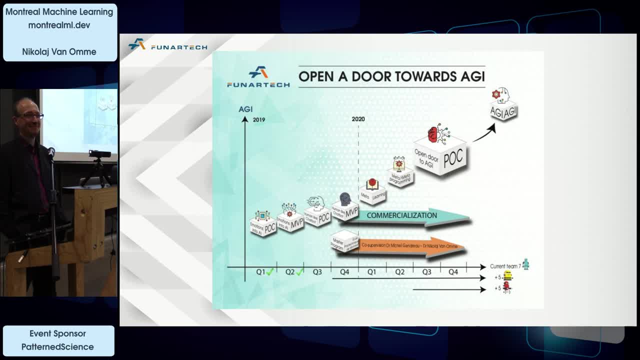 Yes, So thank you so much for your presentation. I'm interested in the part of emotions. Mm-hmm, You said it's very hard to do it using, All right, the ML. how would this be possible with a work? 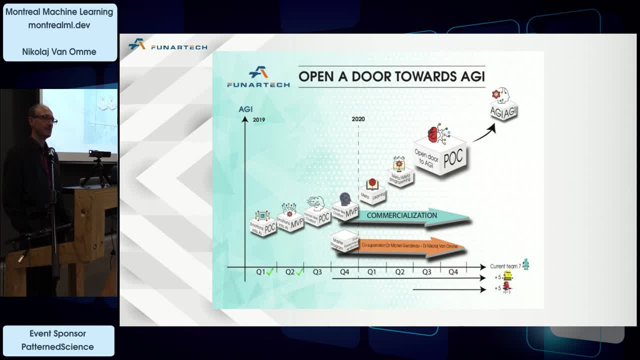 I know because I worked on this film. The main issue we had was about getting training data for ML And what we did. we tried to kind of go around and use some kind of hard code without taking it. It wasn't really that I said there's. 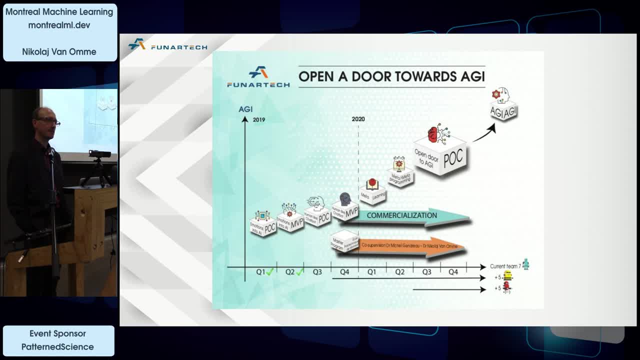 some kind of research existing. some other universities did collect their own labeled data. They write some text like novels and put a label about angry, that kind of Well, that's the main issue for me, Otherwise it's easy. 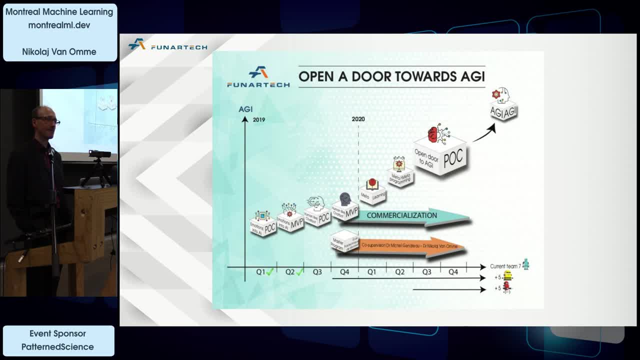 If we have labeled data sharing, it would do great. Yes, except that you need data. that is huge. I mean you need more data than there are atoms in the universe. I would say, If you have all the data, then all the problems are solved. 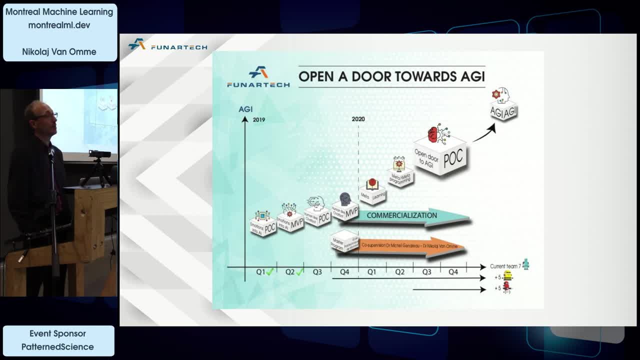 And then machine learning is working pretty well. Yes, but this is not the case And it will never be the case. What about reinforcement learning? We are also using reinforcement learning, but not only So. the key is to use all those tools and to put them together. 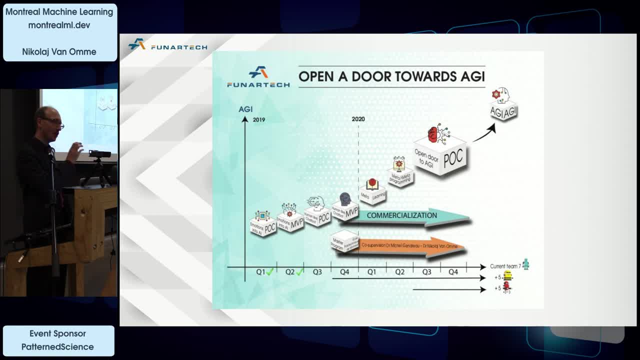 If you know the advantages and disadvantages of all the tools and you know how to combine them so that you can combine the advantages, you go way further. You didn't give us more details. No, I didn't, because this is proprietary. Yes, 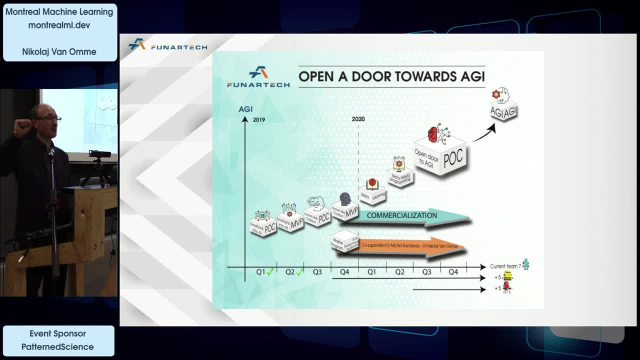 No, the thing is a few years ago I came and I knocked on doors And I was a crazy guy. No one believed me. So I have a company now and I'm building it and I'm selling it. 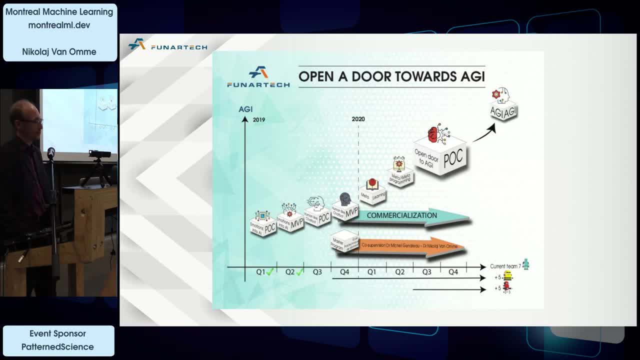 And then next year we're going to go back to university And probably we're going to give some back and we will write some articles, But for the moment, no, it's proprietary. Thanks for the presentation. You mentioned that your system autonomously changes emotions. 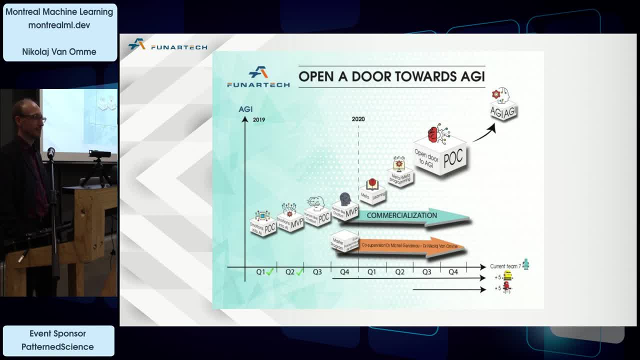 Yes, And doesn't get berserk. Yes, And you said it's controlled. Yes, So is the control external or is it built into the system? That's the first part of the question. What do you mean by external? I mean it's inside the system. 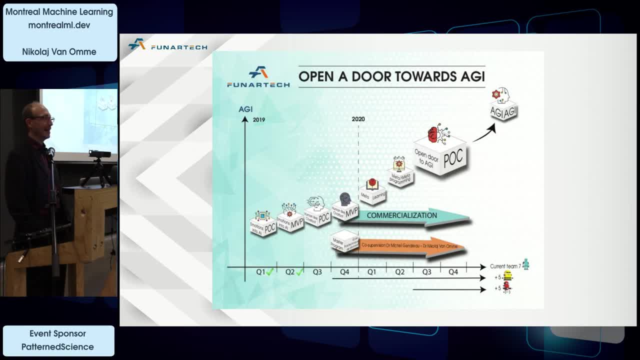 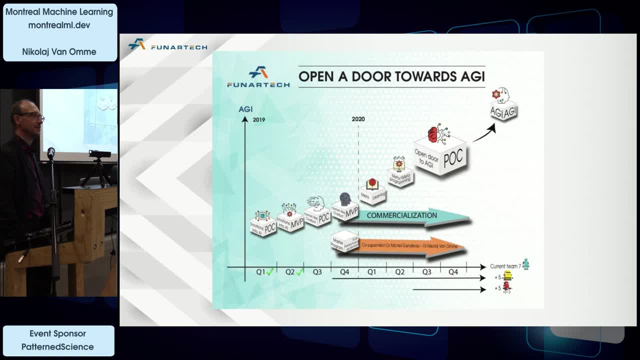 I mean, I would like to know what you would So A you say that a system is at a particular emotion. Yes, Let's say it's a chatbot, Mm-hmm, It's a group, So there's an angry customer. 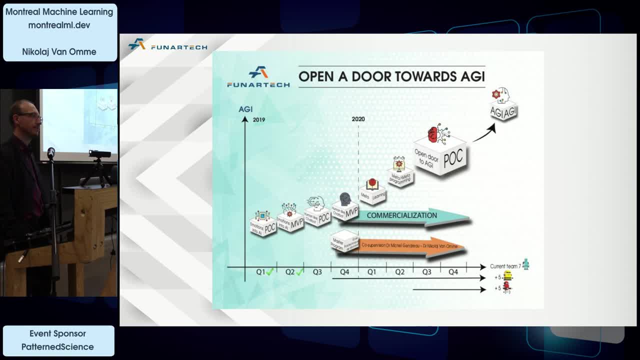 Yes, And there's this chatbot that is assimilating. it is sensing that the customer is angry And it could possibly react in a way that a customer representative would a human customer representative. If it is to emulate a human customer representative, it would react in a way that a human customer. 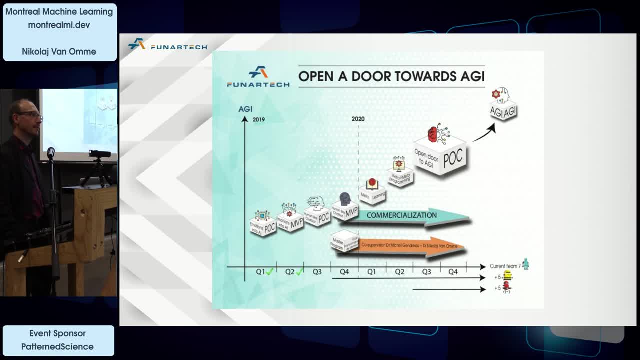 representative would. So if it is to emulate a human customer, it would possibly first try to understand what is the source of the problem and try to address the root cause of the problem, Right, Mm-hmm? And in course of it, you are programming submissive states into the system. 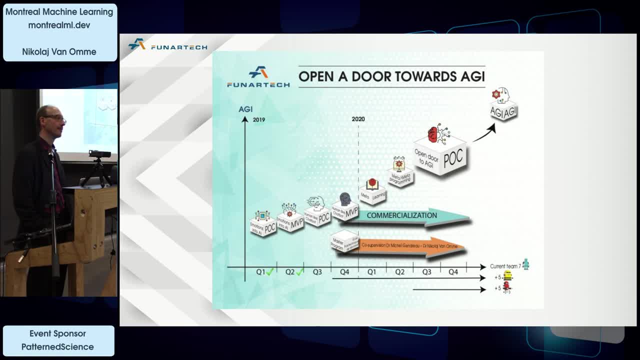 Is that right? You have to. Yes, I mean we are. Well, we are combining all those tools, Right. So you move from one state to the other state and it is more submissive in the sense that you can, You can. 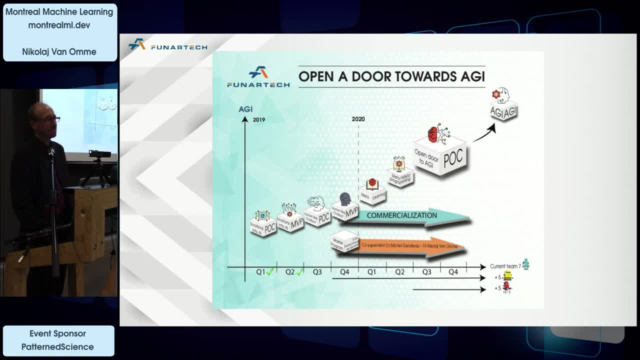 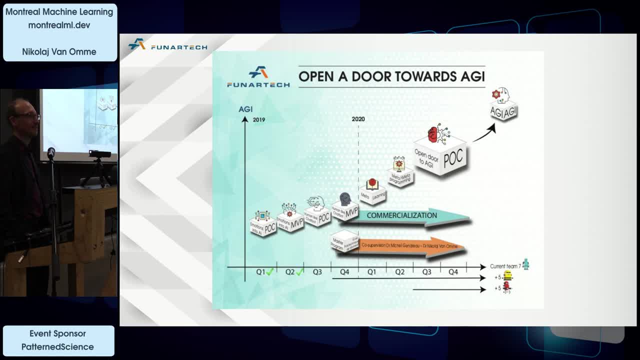 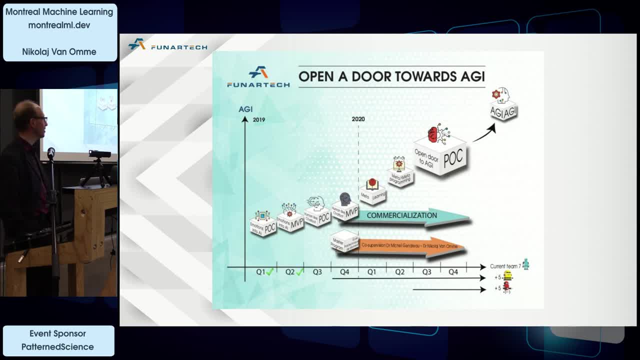 So actually I'm going to give you something more. Our system can also find out by itself what emotion is. Not in the sense that it knows what emotion is, but it detects what an emotion looks like and how to mimic it. We have no idea what emotion is. 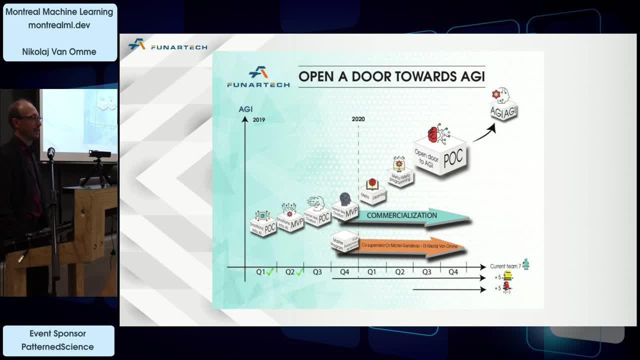 But we mimic emotions. What was your question? again, Sorry. So how do you say that you are moving the? Okay? Well, how can I explain this without giving too much away? I would say that if you are interested, let's talk. 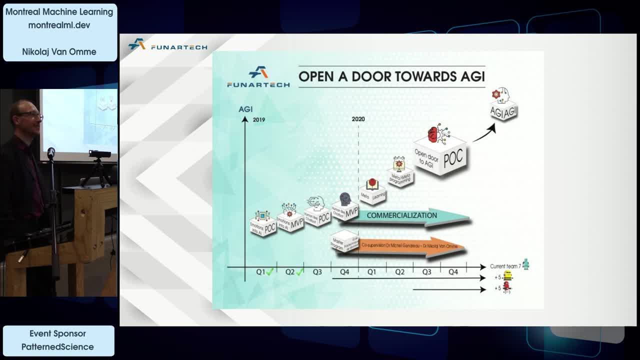 But probably, if I say too much, then I mean there are lots of clever people here in the room And what we do is not that exceptional. I mean, Okay, probably I look forward to your kind of project, Thank you. So one last question.